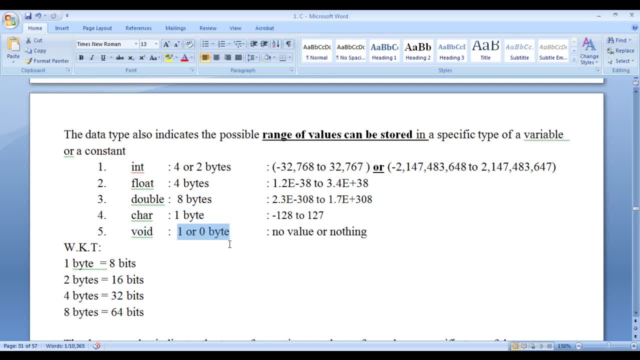 will be allocated. For character type of data, 1 byte of memory location will be allocated. For white type of data, 1 or 0 byte memory location will be allocated. We have seen in the previous video tutorial in the code blocks. we have seen that for 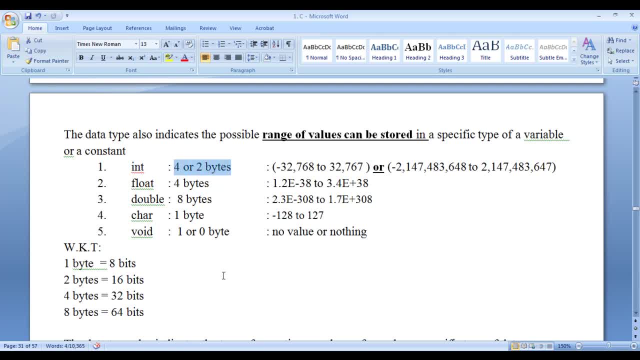 integer type of data: 4 bytes of memory location will be allocated. For float type of data: 4 bytes of memory location will be allocated. For double type of data: 8 bytes of memory location will be allocated. For character type of data: 1 byte of memory location will be allocated. 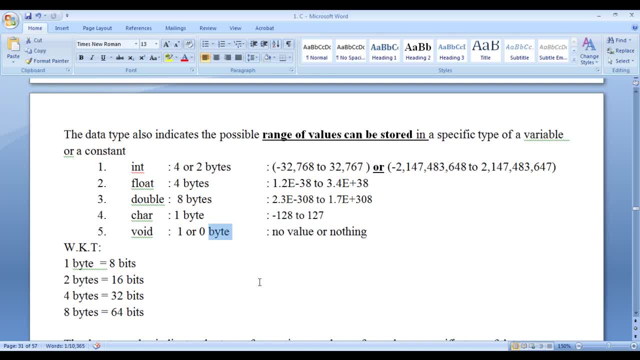 For white type of data, 1 byte of memory location will be allocated. Data type not only indicates the type of data and the amount of memory to be allocated for a specific type of data. data type also indicates the possible range of values can be stored in a specific type of variable or a constant. 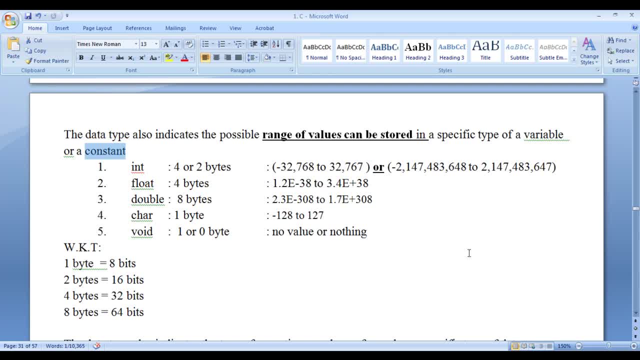 What is a variable or a constant? You can think like variable or a constant is a chunk of memory, a memory location. Data type determines the minimum and a maximum value possible to store in a specific type of variable or a constant. If int is of 2 bytes, then a variable or a constant of type int can have 65,536 numbers. 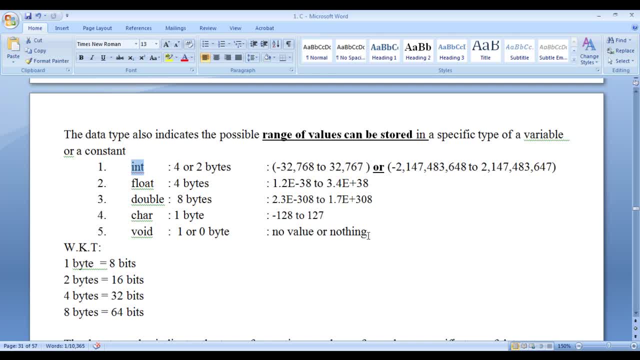 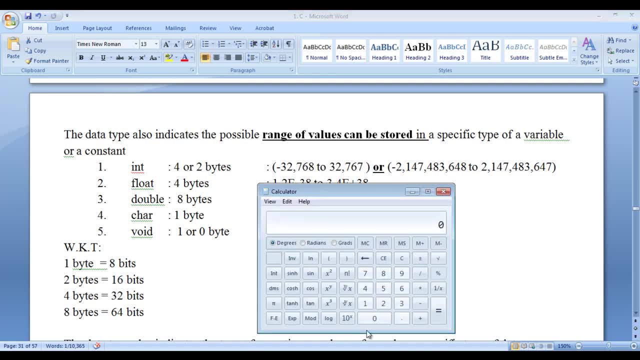 How do we say 65,536 numbers only If int is of 2 bytes, that means 16 bits. we know that binary number system base is 2, raised to the power of 16 is equal to 65,536. 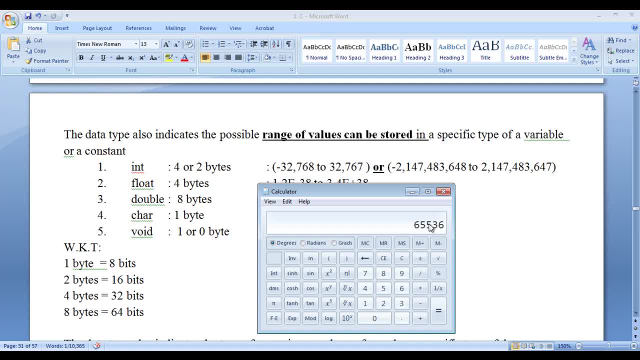 Right, That is the reason I am telling. a variable or a constant of type int of 2 bytes can have 65,536 numbers. If I divide it by 2, it is equal to 32,768.. The minimum value possible to store is minus 32,768. 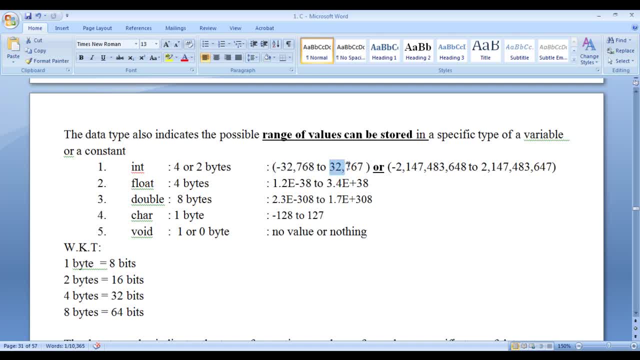 And the maximum value possible to store is 32,767.. If you count from minus 32,768. That is the reason I am telling- From 32,768 to plus 32,767, it is going to be 65,536 friends. 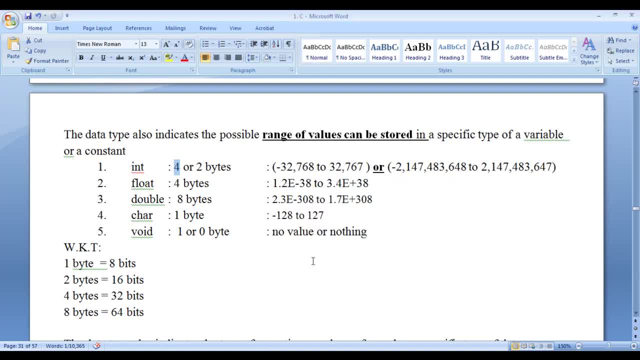 Similarly, if int is of 4 bytes, then a variable or a constant of type int can have 4 billion plus values or 4 billion plus numbers. How do we say 4 billion plus numbers If int is of 4 bytes? 4 bytes means 32 bits. 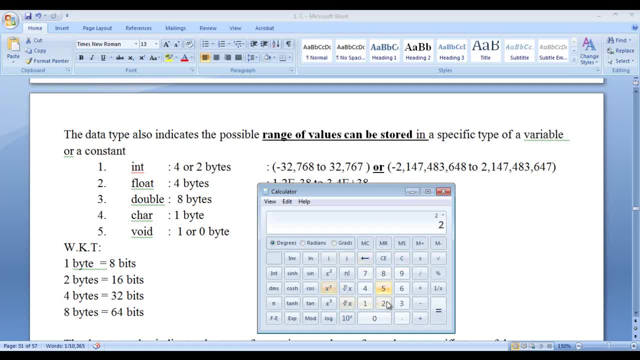 So here I say: 2 raised to the power of 32 is equal to 4 billion plus. you can see that If I divide it by 2, it is going to be 2147483648, so it's a 2 billion plus number. 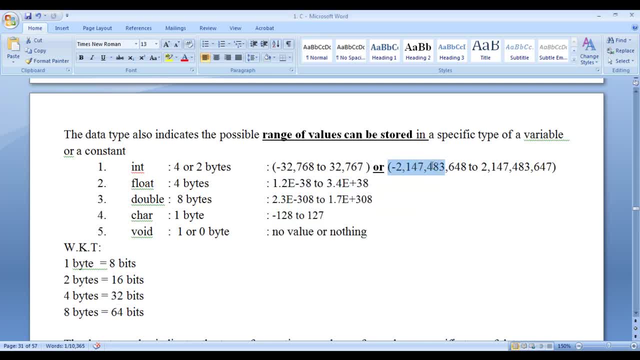 The minimum value possible is minus 2147483648.. And the maximum value possible is 2147483647.. If you count from minus 2147483648, it is going to be 2147483648.. So here I say: 2 raised to the power of 32 is equal to 4 billion plus. you can see that. 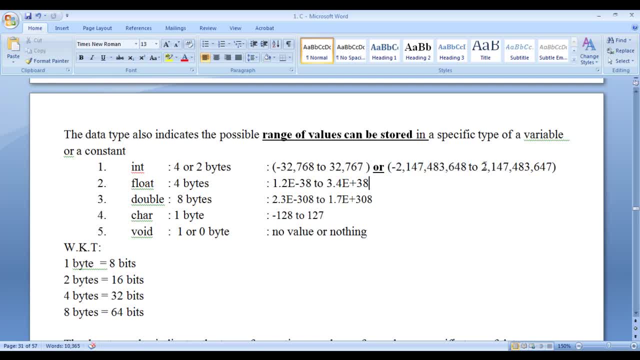 So from 2147483648 to 2147483647, it is going to be 4 billion plus. Minimum is minus 2 billion and maximum is plus 2 billion plus. If a variable or a constant is of float type of data, then the minimum value possible to 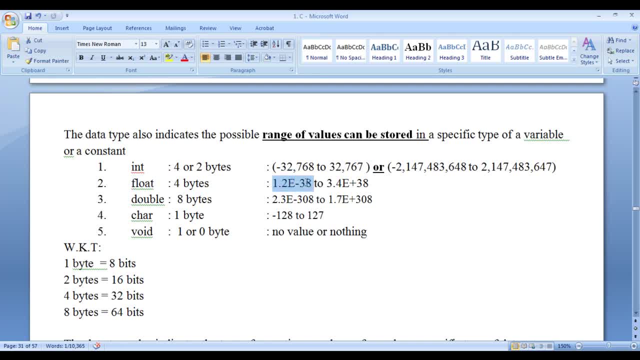 store is 1.2e – 38. And the maximum value possible is 3.4e plus 38.. If a variable or a constant is of type double, then the minimum value possible to store is 2.3e minus 308 and the maximum value possible is 1.7e plus 308.. 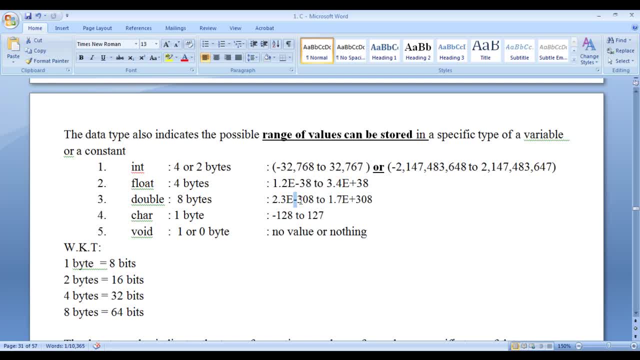 You can see the difference here: Minus 38 minus 308, plus 38 plus 308, there is a lot difference. you can see If a variable or a constant is of character type of data. the minimum value possible is minus 128 and the maximum value possible to store is 127. 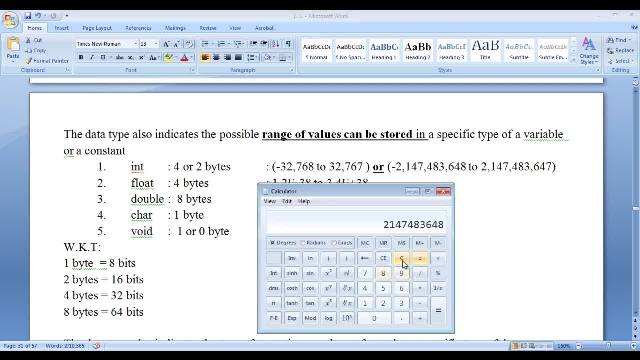 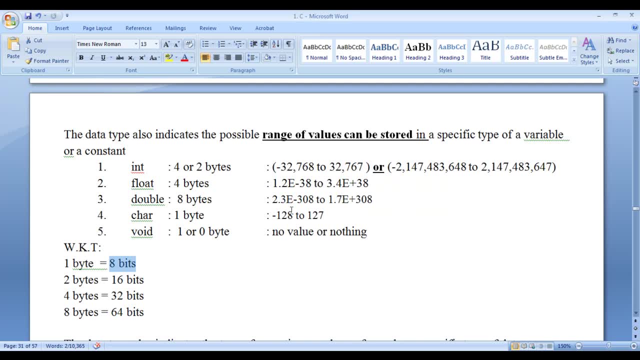 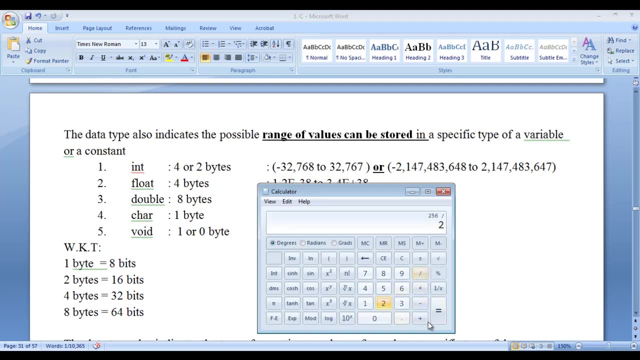 One byte is equal to 8 bits. Let me take the calculator clear. this 2 raised to the power of 8 is equal to 256.. 256 values possible to store in a variable or a constant of character type. If I divide it by 2, it is going to be 128. 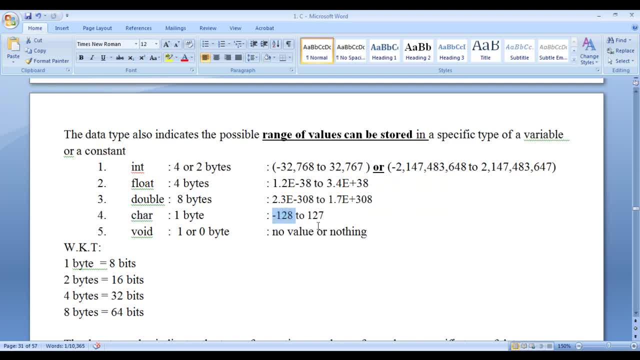 So minimum value possible is minus 128 and the maximum value possible is 126.. If you count from minus 128 to 127, it is going to become 256.. Let's have a demonstration and display the minimum value possible to store and the maximum. 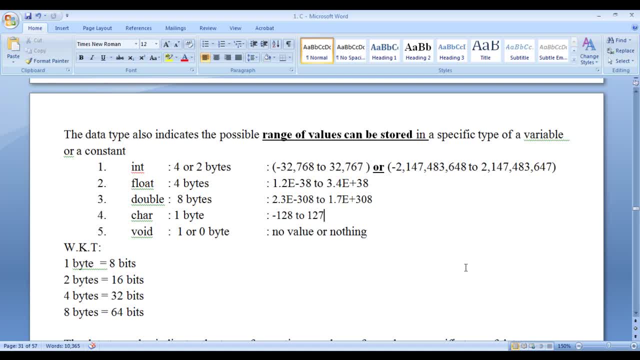 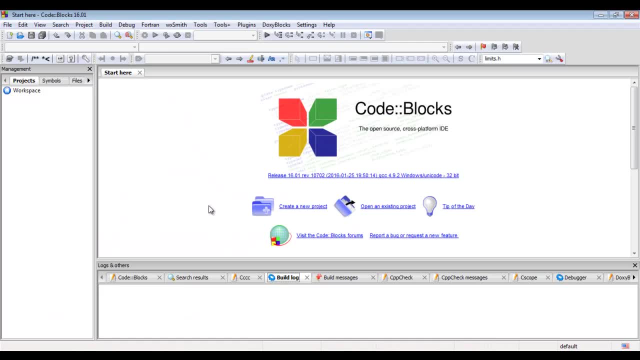 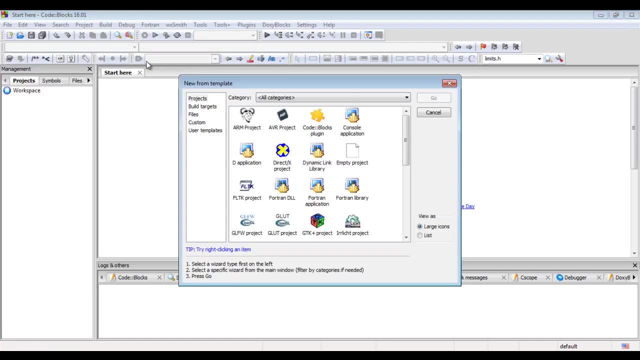 value possible to store in a specific type of a variable or a constant. Let me minimize the MS word. I double click on code blocks to launch the code blocks IDE. You can see that the code blocks IDE got launched. I'm going to create one new project by going to file, say new, click on the project. 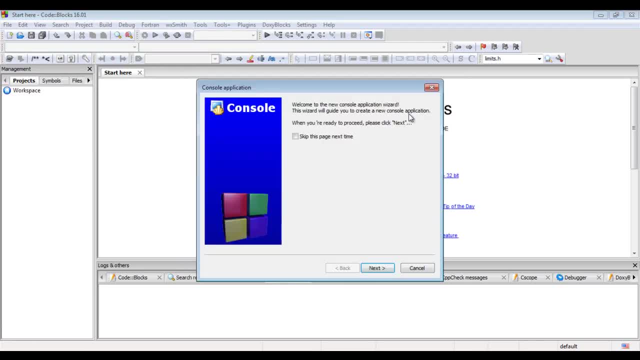 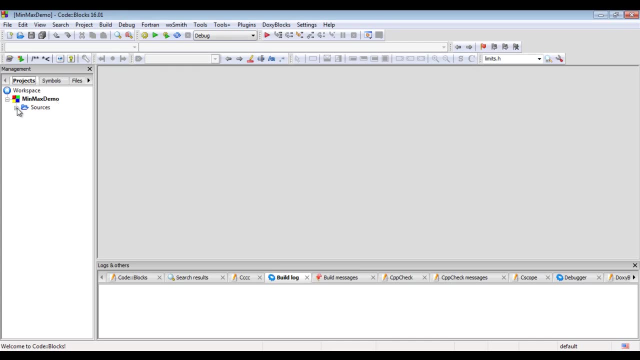 I select project, say console application, say go, and I say next select C language, say next, and I give the project title as minmaxdemo and I say next, say finish. You can see that minmaxdemo project is open. I click on the plus sign, double click on mainc to open it. 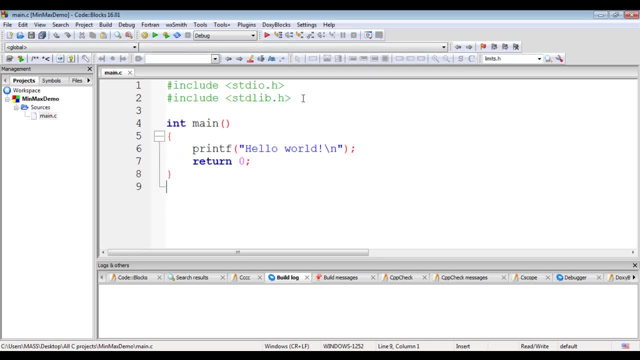 I zoom little bit so that we can see the content properly and I select this line of code, say delete. I do not want that code. Now when I say build and run, We know that the hash include preprocessor directive is going to direct the preprocessor. 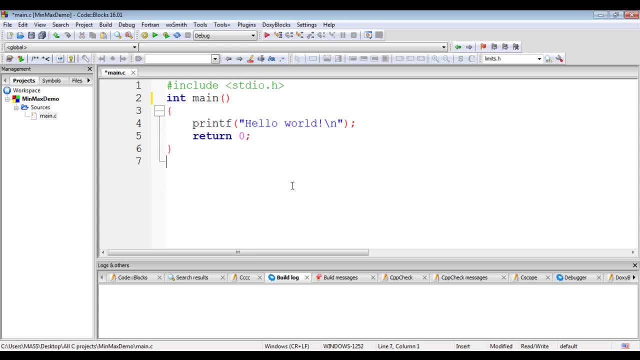 to include stdioh in the mainc file. stdioh is going to be included in the mainc file and then the program execution begins at main function. The printf function displays hello world exclamation mark and moves the cursor to the next line. 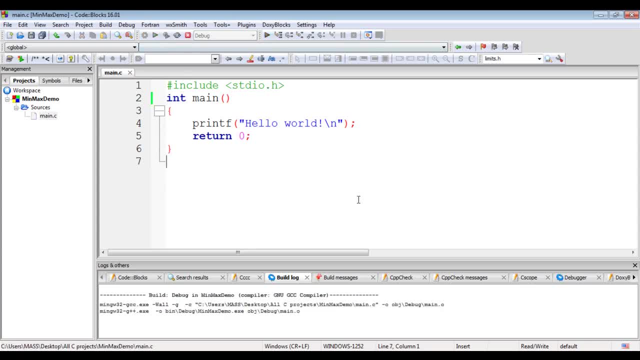 and zero will be returned to the operating system. If I say build and run, you see, hello world. exclamation mark got displayed. I hit enter. Now we display min and max values. okay, Here I say int min equal to. if I say build and run, you can see we are seeing int min. 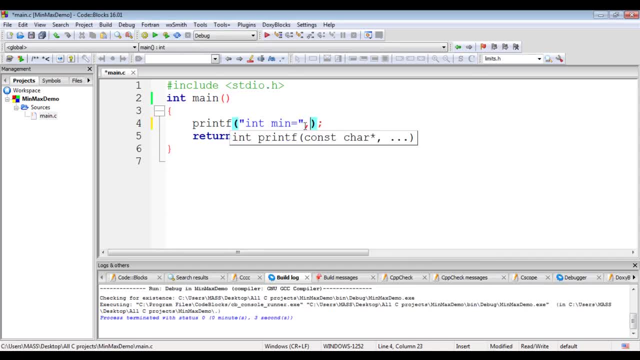 equal to. I hit enter and we are going to take help of some constants available already in the library, that is int underscore, min, min. If I say build and run, You see an error, That Int min is undeclared. It is telling that I don't know what is the meaning of int min. 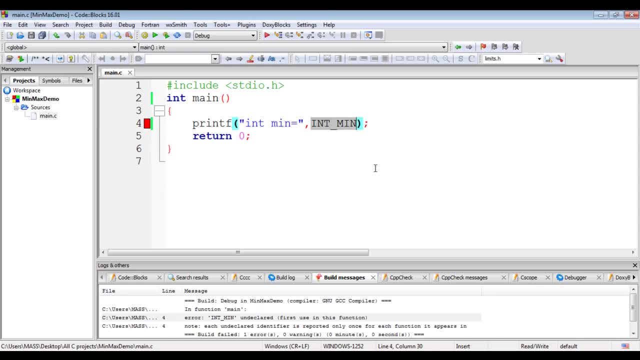 Where is it? int min is available in another header file, that is limits dot h file. I have to include that to use this constant Here. I say hash, include limits dot h, close In the limits dot h. we have this macro, int min. 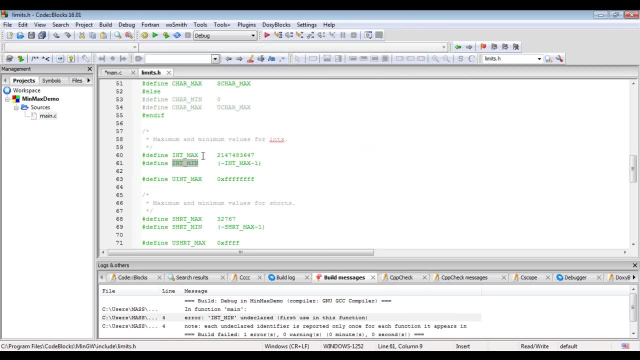 If I right click, say find declaration for int min, It goes to the limits dot h file. That is the reason I have included here limits dot h to use int min in my program. If I say build and run system is displaying int min equal to. 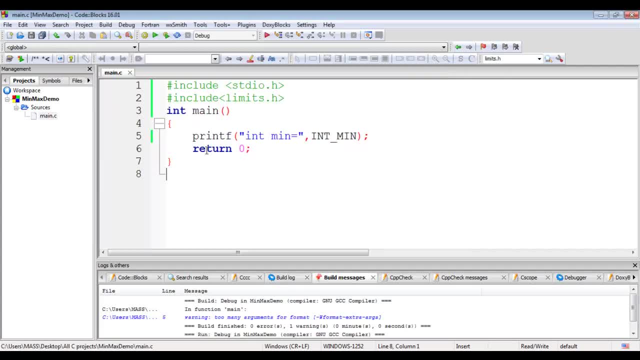 There is no minimum value, right, I hit enter. How do we display the value of int min? We need to take help of format specifiers that we learned in the previous video tutorials. Here I say percentage i And then I say backward slash. 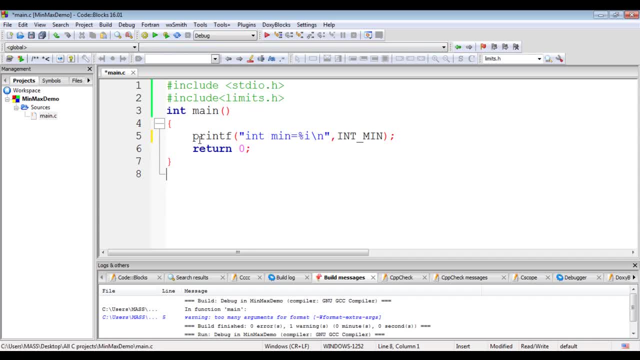 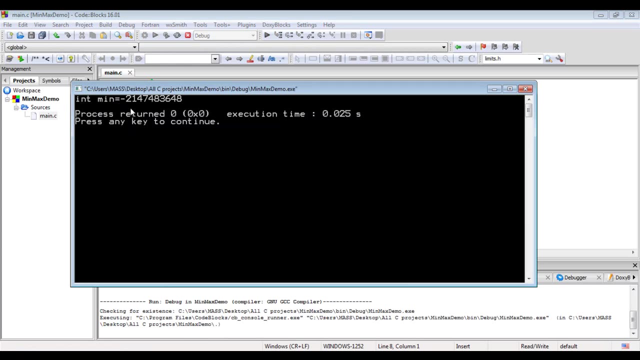 This time, when I say build and run, the printf function is going to display int min equal to This place is going to be replaced by the value of int min And then backward slash n moves the cursor to the next line. If I say build and run, you see int min is equal to minus 2147483648. 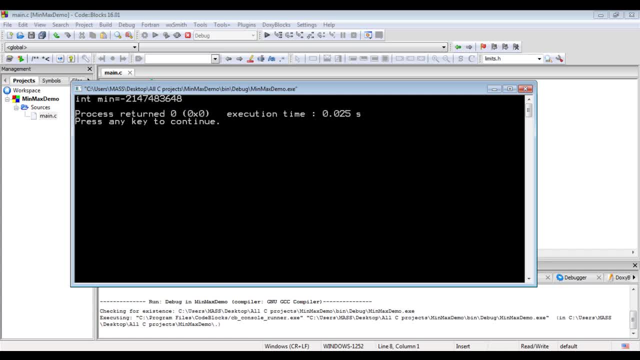 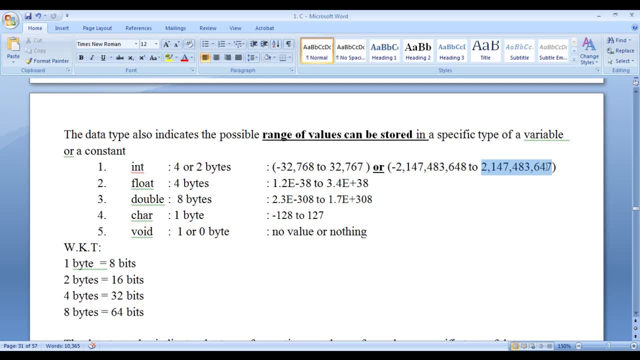 That is the minimum value possible for integer type of data. So that's what I have here, Minus 2147483648.. That's it. We can also display the maximum value possible. I go back to word blocks. I hit enter here. 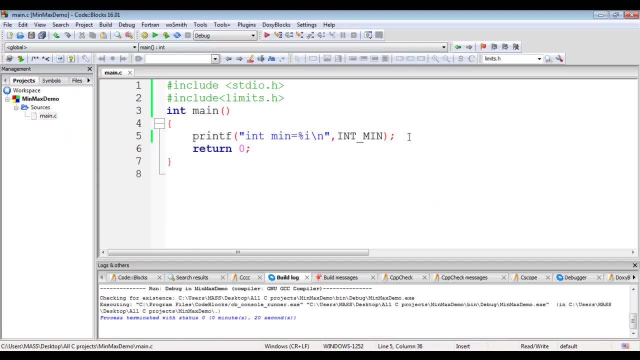 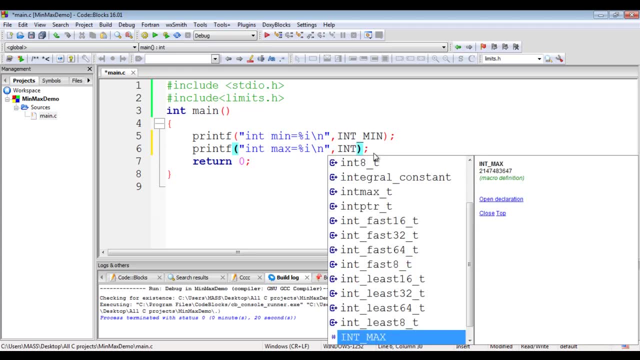 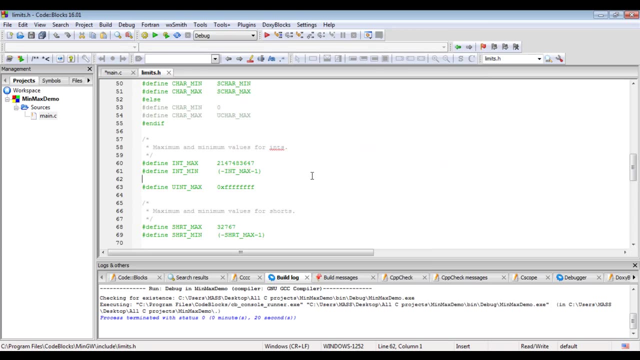 I'm going to copy this line of code and paste down Here. I say int max and this place I'm going to replace int underscore max. If I right click find declaration for int max, it is available in the limits, dot h. Its value is 2147483647. 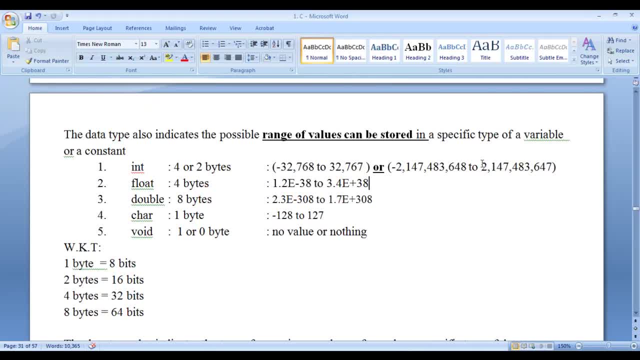 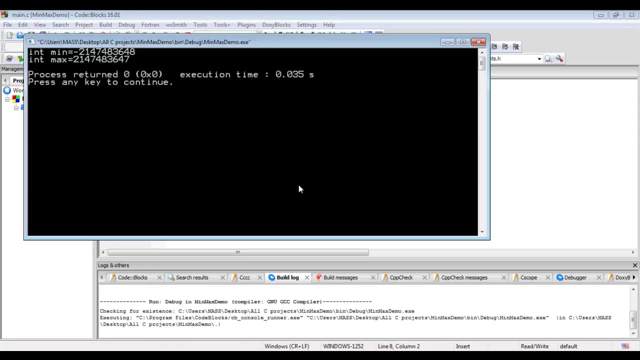 That is 2147483647.. That's it. That is the max value This is going to be displayed. Okay, Let me close it If I say build and run, you see, int max is 2147483647.. That is 2 billion plus value. 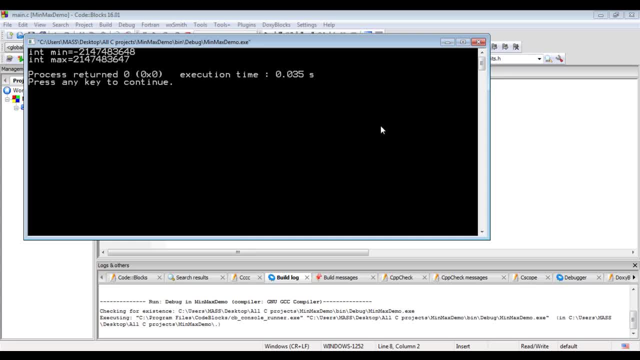 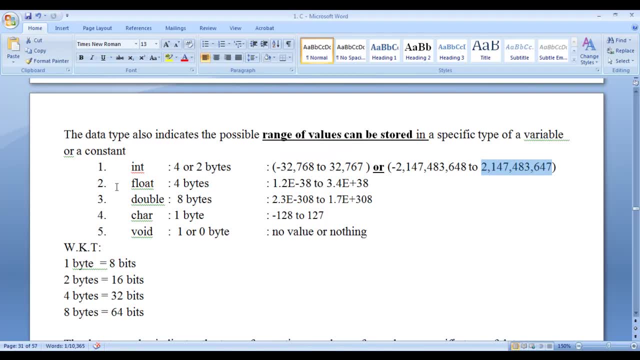 I hope you guys have understood how to display the min and max values of integer data type. I hit enter. Now we display the min and max values for float. Let me go back. I'm going to copy this line of code. I hit enter. 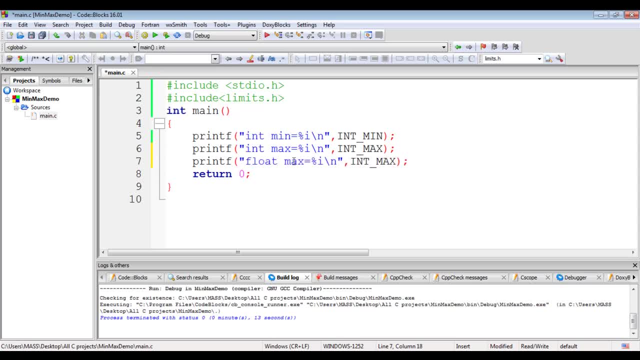 I hit enter and paste down. Here I say float min Instead of %i. I use %e because I want to display the float min in the scientific notation, So I'm going to use flt underscore min constant. If I say build and run, we get an error message that I don't know. what is the meaning of float? 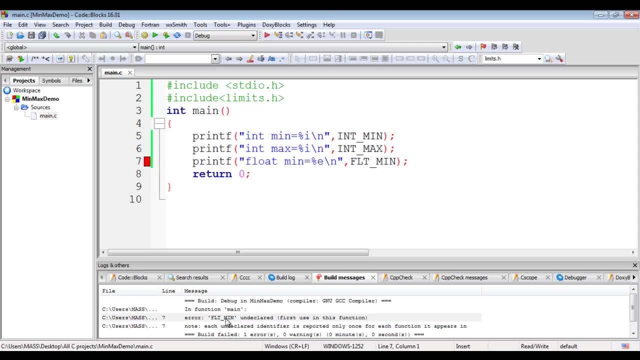 min Float min undeclared. It is telling error, Right, Because min flt min constant is not available in limitsh. It is in another header file That is floatsh file. I'm going to include that Hash. include floath header file This time. 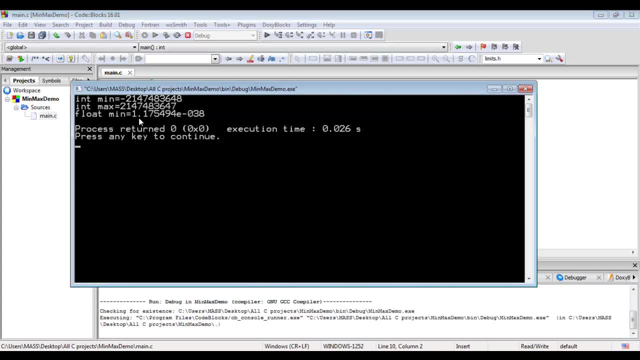 if I build and run, you see, float min is 1.175494.. You can round up it to 2.. 1.2e-0.38.. 0 is not important here, You can just say 38.. That is actually the minimum value of float datatype. 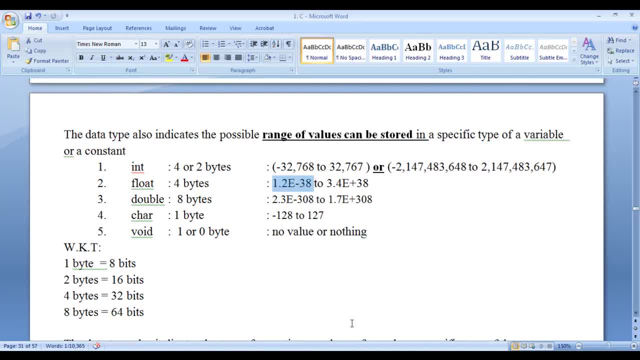 You can see that 1.2e-38.. You can say 1.2e-38.. This and that both are same. If I hit enter and I go back here and now I display the max value. I'm going to copy this line of code. 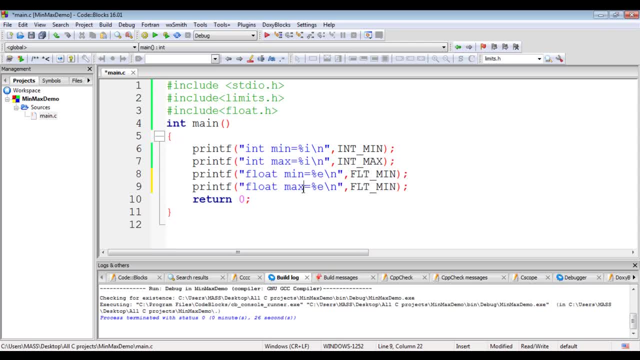 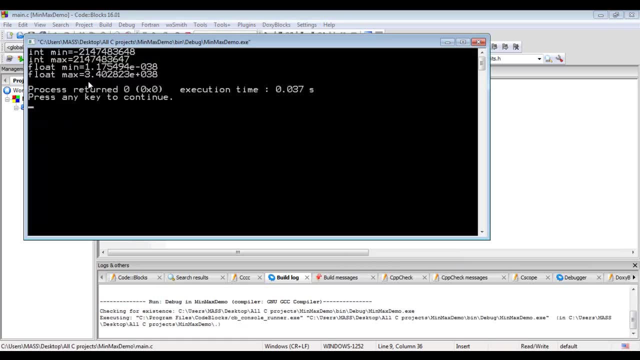 and paste down Here. I say float max and I use here float max. And if I say build and run float max, And if I say build and run float max, And if I say build and run float max, You see the max value is 3.4 plus 38.. Right, I hit enter. That is what we have. 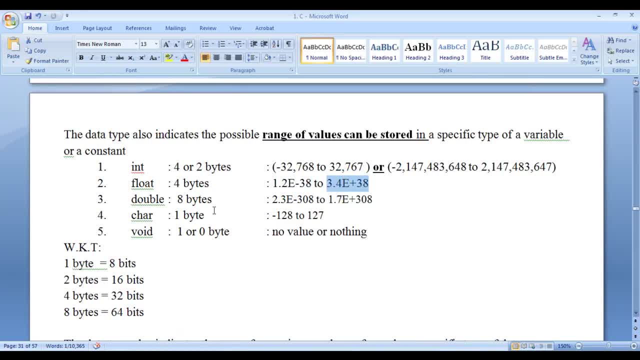 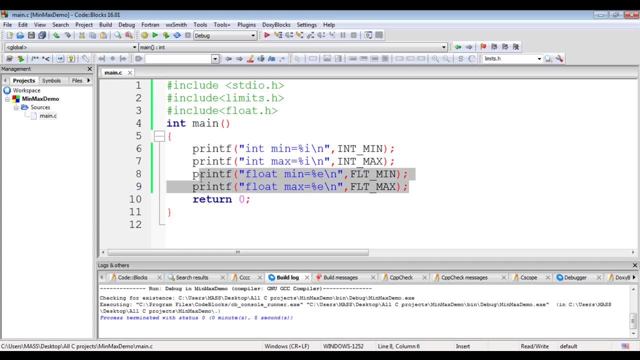 here 3.4e plus 38.. We can display now the min and max values for double datatype. Go back and I'm going to select these two lines of code, Copy and paste down. And I change here: d-o-u-b-l-e-double. Here also I change d-o-u-b-l-e-double, And here also I change. 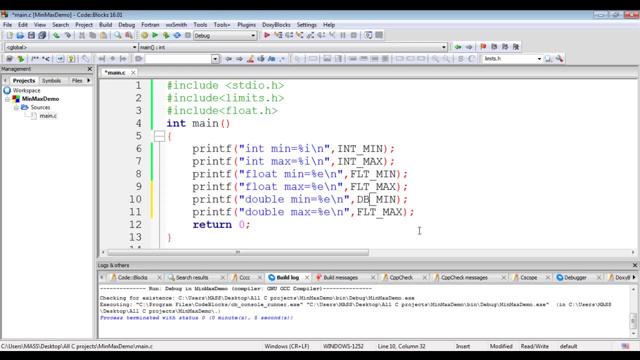 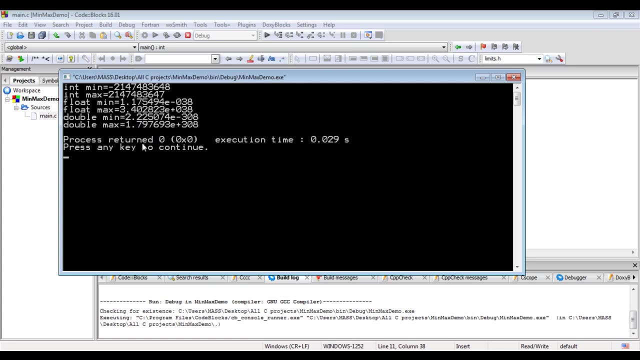 d-o-u-b-l-e-double Instead of flt. I use here d-b-l and I say here d-b-l. d-b-l means double. If I say build and run. you see, the minimum is 2.2 minus 308 and maximum is 1.7. 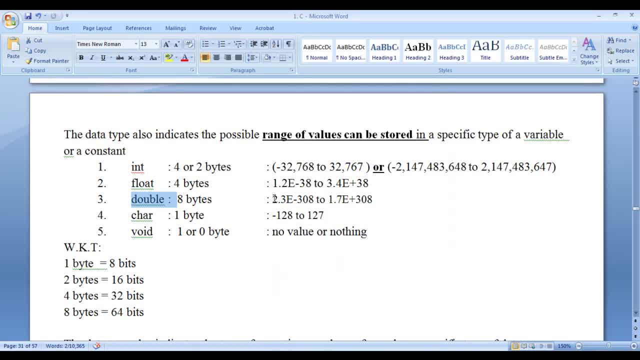 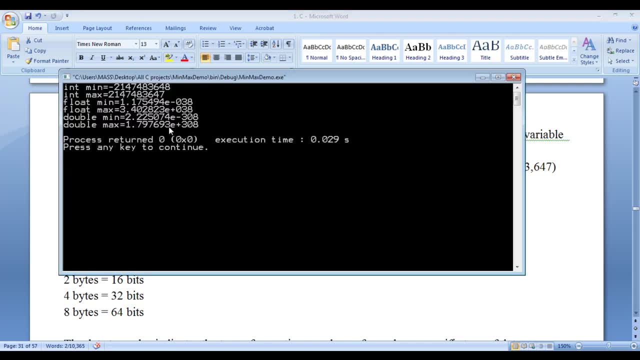 plus 308.. That is what we have here: 2.3 minus 308 to 1.7, 308.. Right, That's what we have here: 1.7 plus 308.. That is what we have here: 2.3 minus 308 to 1.7, 308.. Right, That's what we have here: 1.7. 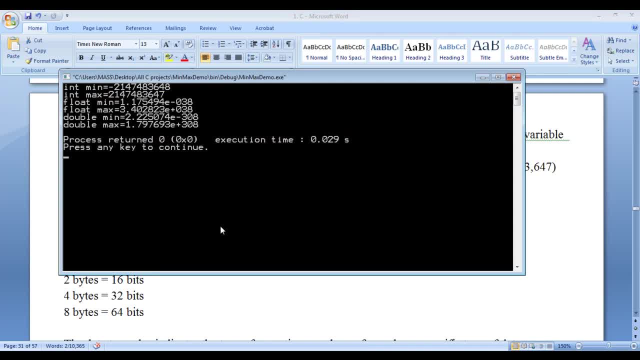 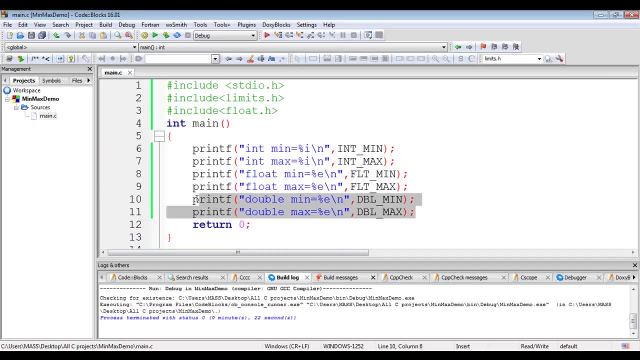 plus 308.. That is what we have here: 1.7 plus 308 to 1.7, 308.. We have displayed the possible min and max values for double data type. Similarly we can display for character data type. Now I'm going to copy these two lines of code and paste down Here. I say char. 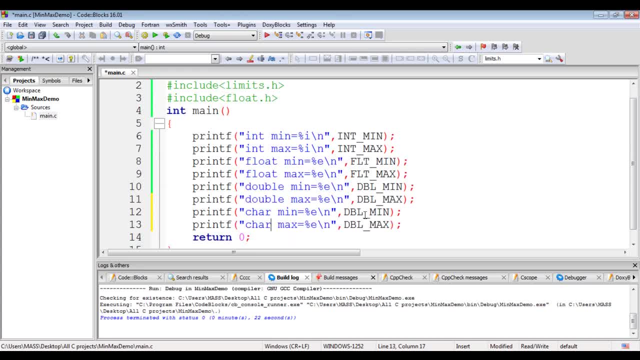 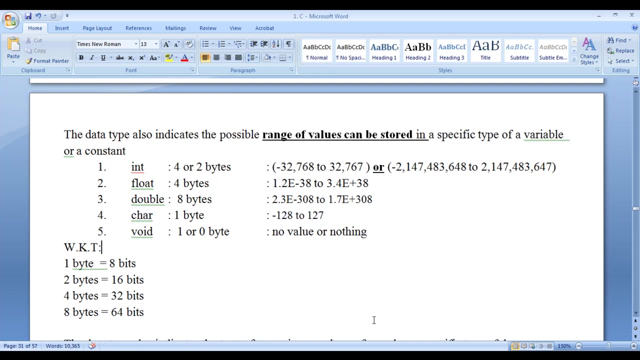 min and char max. And this place I say char min and here I say char max. Here I use plus percentage i, Percentage i. If I say build and run, you see last outputs- char min is minus 128,, char max is plus 127. That's what I told here. Char min is minus 128, maximum is 127. This is how. 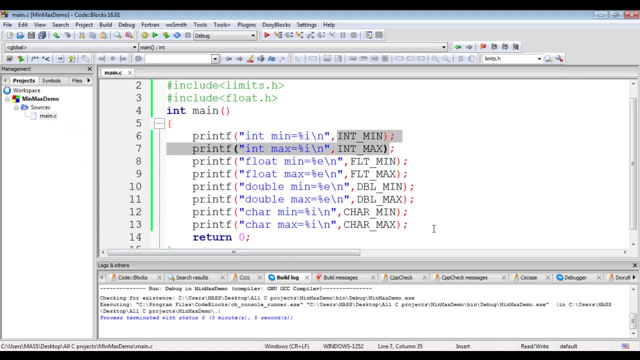 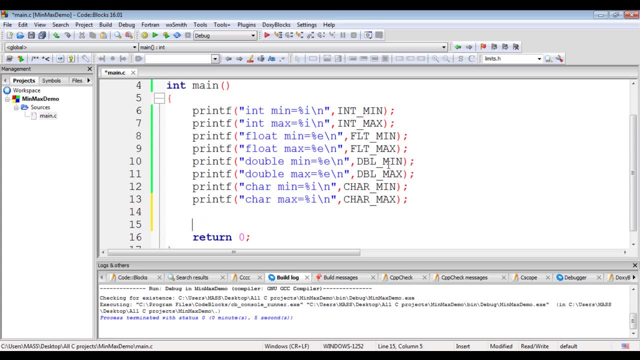 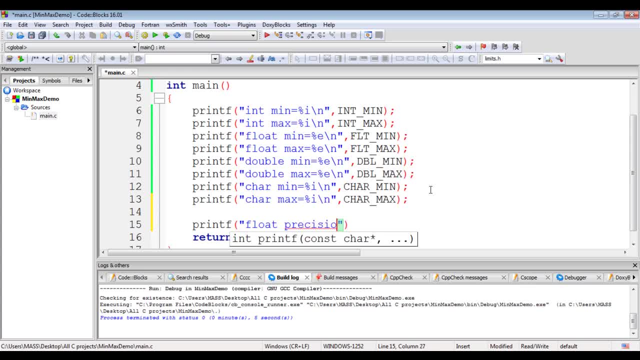 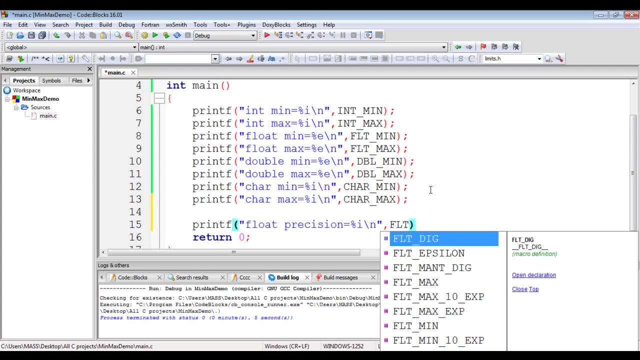 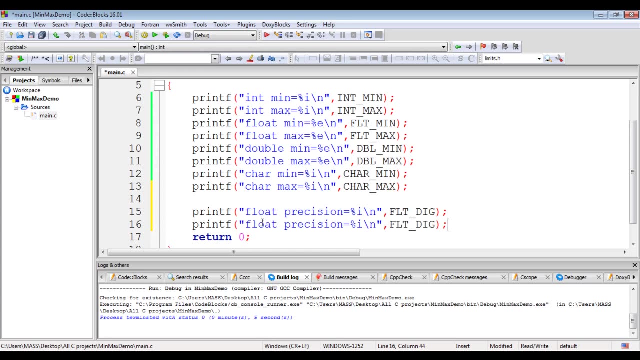 I just say float precision. when precision is equal to percentage, i backwork slash n comma, fold underscore semana semicolon. I am going to copy this line of code and paste down. This is going to be dou ble, double. And here I say DBLdig. and this is my code. 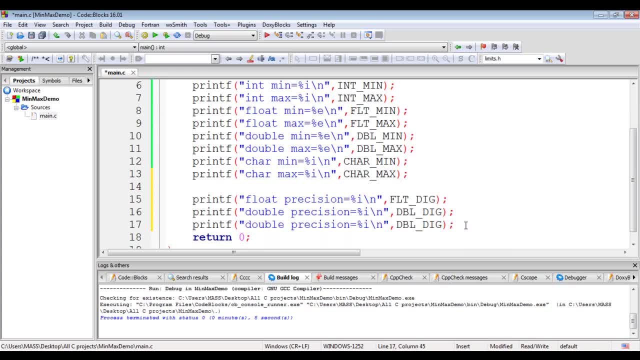 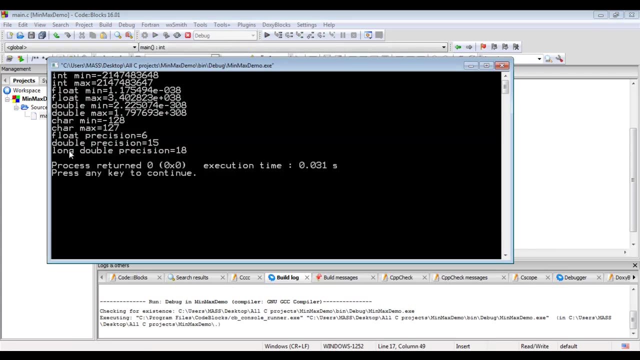 and copy this line of code and paste down. say here: long double. we have long double data type. I discuss about long double and all later, and here I say l d bl did yes. if I say build and run, you see float precision is 6, double precision is 15. long double precision is 18. 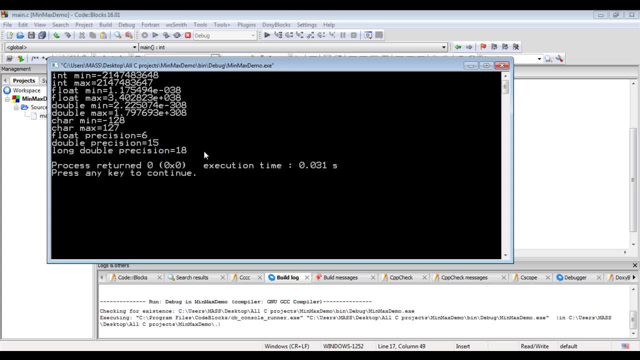 that means: float can store 6 digits after the decimal point. double can store 15 digits after the decimal point. long double can store 18 digits after the decimal point. a very high accurate result you can get using the long double variable or a constant. I hope you guys. 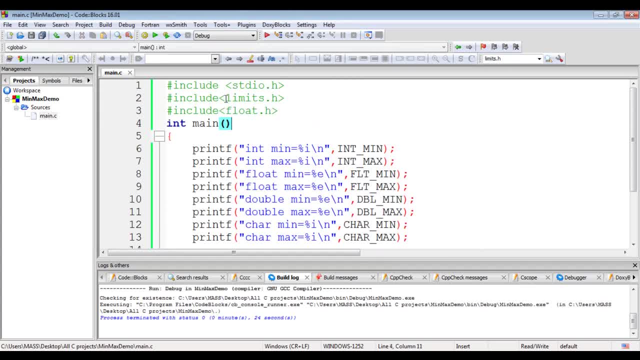 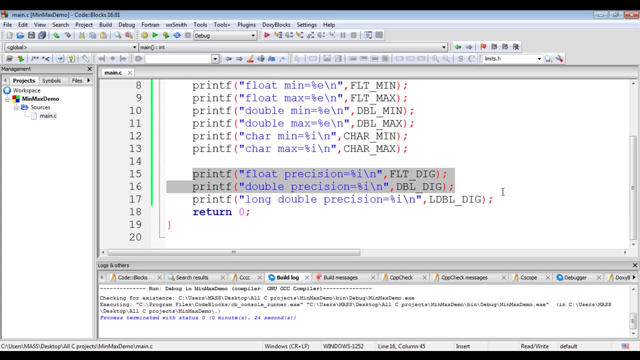 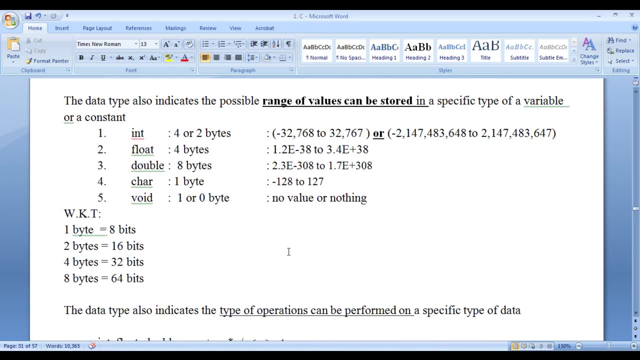 have clearly understood how to use floath header file, limith file, how they are used to display min and max values, how they are used to display the precisions of real type data. one more point I want to discuss. data types also indicate that if you want to display the precision of real type data, you need to 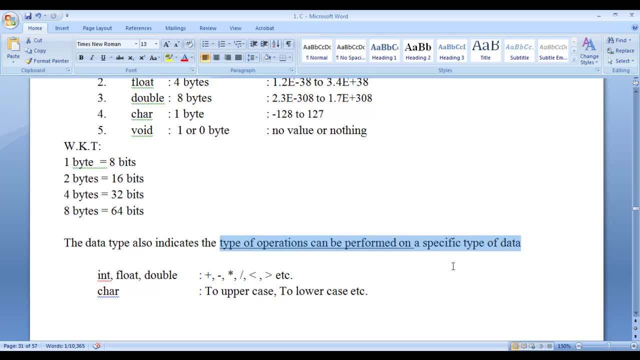 indicate type of operations can be performed on specific type of data. that means on integer, float, double. we can perform addition, subtraction, multiplication, division. we can even check less than greater than right. we can perform on characters or strings: uppercase to lowercase operations. we can convert a character to uppercase. we can convert a character to a lowercase. 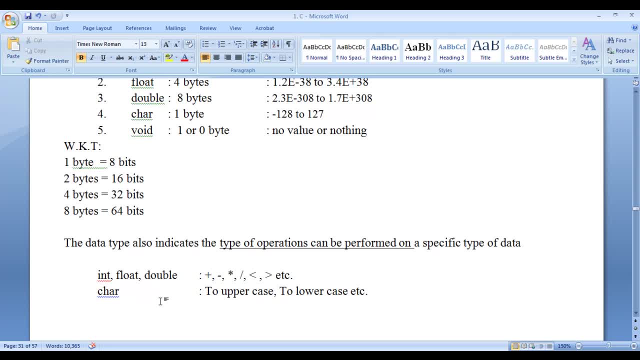 but we cannot perform two uppercase or two lowercase operations on integer numbers or numbers actually, because they are not valid. we cannot convert a number to a uppercase or lowercase. we can convert a character to an uppercase or lowercase. so two uppercase and two lowercase are valid operations on characters or strings. they are not valid on numbers. similarly, 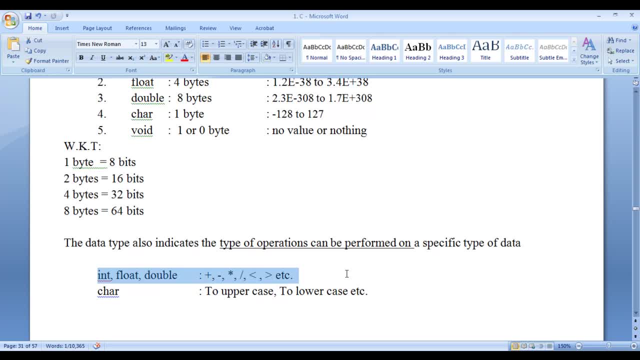 multiplication operation is a valid operation on numbers, but it is not valid on strings or characters, so data type also indicates what type of operations we can perform on specific type of data. what are the things we understood? we understood four important points with respect to data type. data type indicates type of data. second thing we understood: data type indicates the. 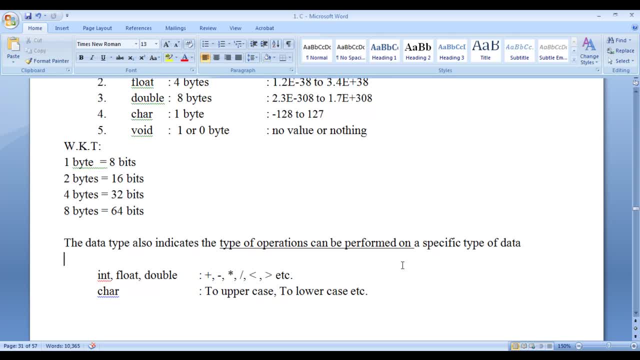 amount of memory to be allocated for specific type of data. third point: what we understood. we understood that data type indicates the possible range of values to be stored in a variable or a constant of specific type. and the fourth point: what we understood: data type indicates what type of operations can be performed on specific type of data. I suggest you people,